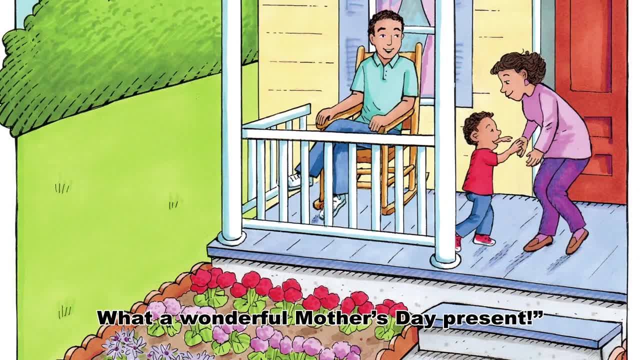 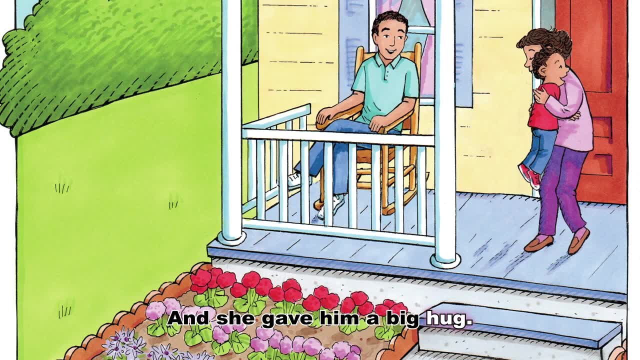 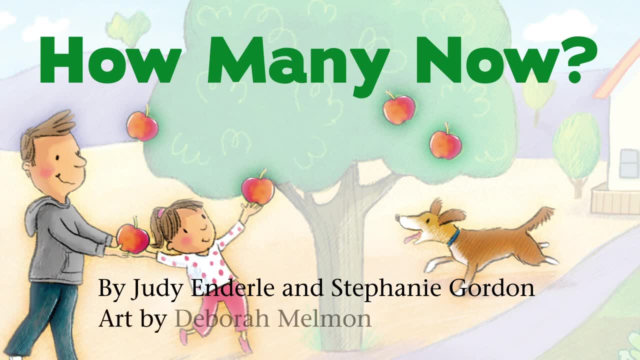 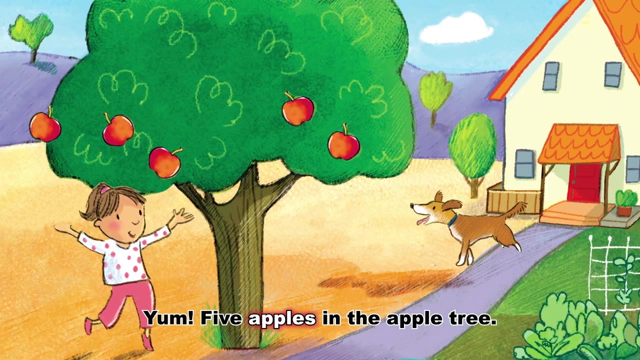 The flower beds are beautiful. Jose, What a wonderful Mother's Day present, And she gave him a big hug. How Many Now? by Judy Enderly and Stephanie Gordon. Art by Deborah Melman. Yum, Five apples in the apple tree. Here's one for you. 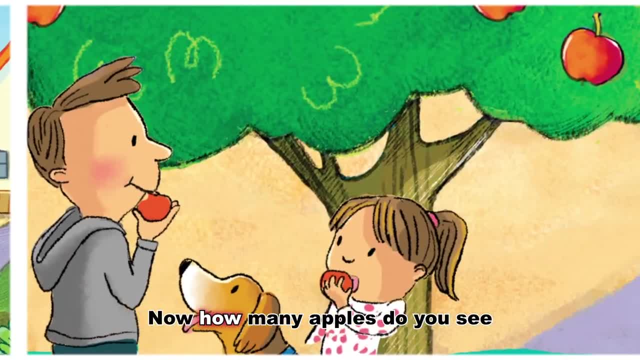 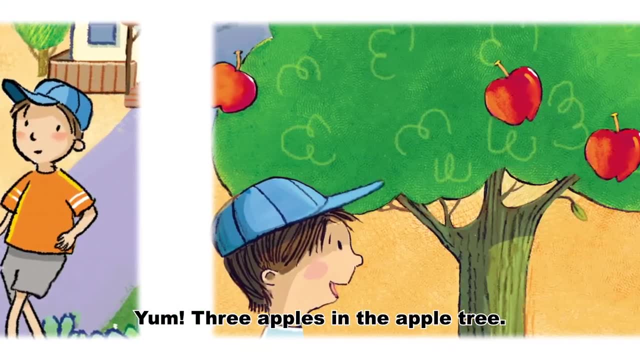 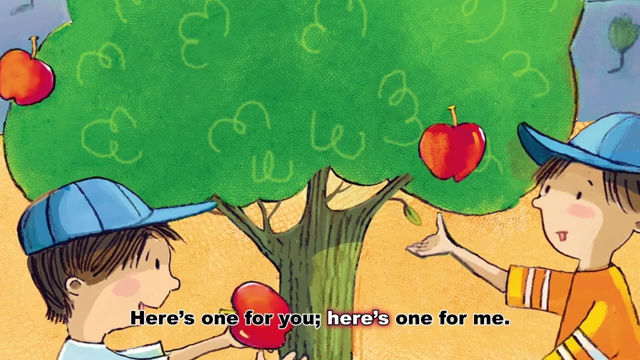 Here's one for you. Here's one for me. Now, how many apples do you see When you are looking up in the apple tree? Yum, Three apples in the apple tree. Here's one for you. Here's one for you. 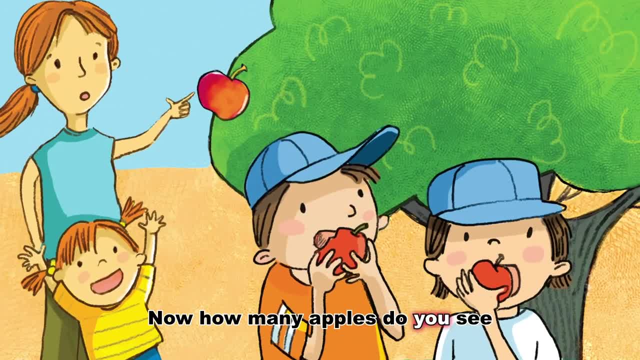 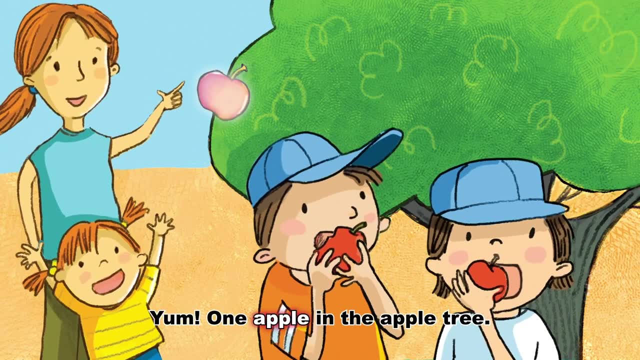 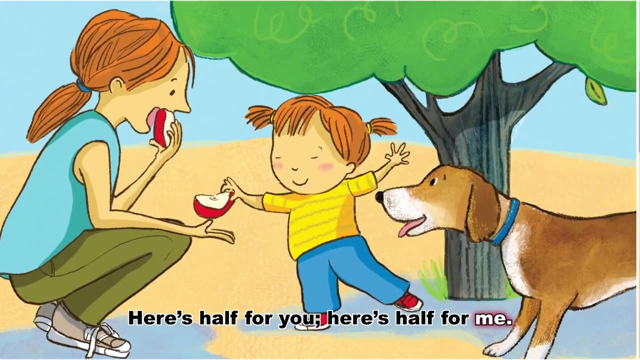 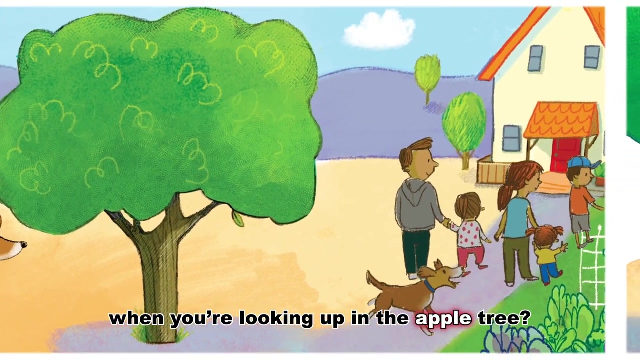 Here's one for me. Now, how many apples do you see When you're looking up in the apple tree? Yum, One apple in the apple tree. Here's half for you. here's half for me. Now, how many apples do you see when you're looking up in the apple tree? 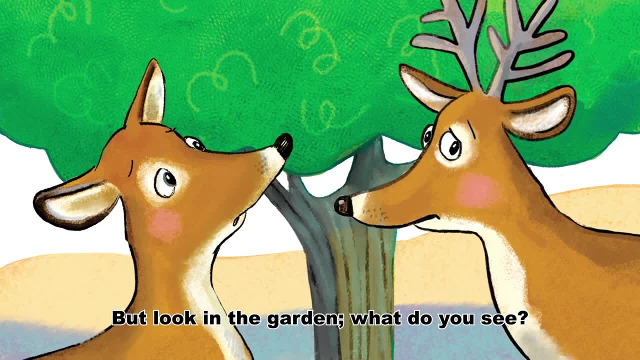 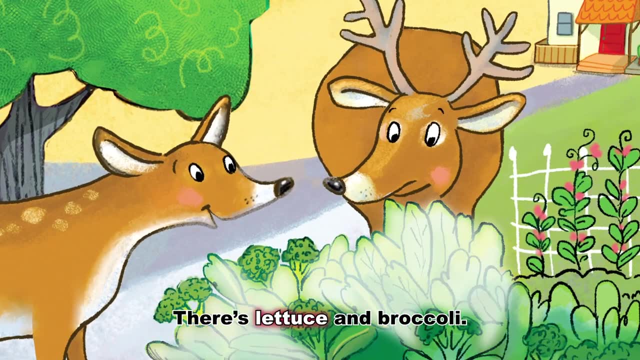 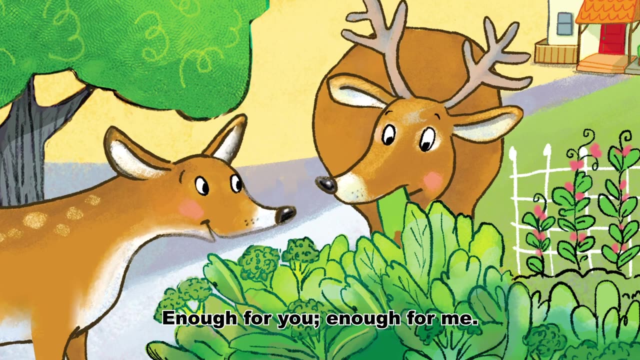 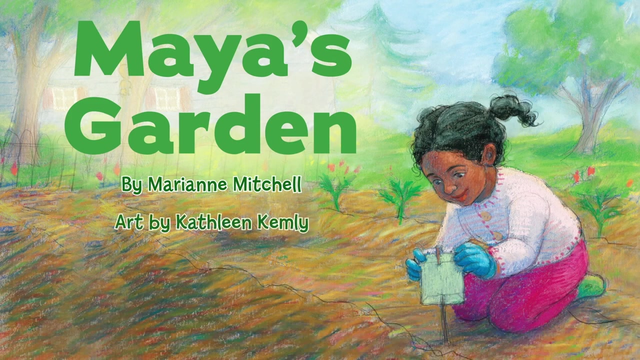 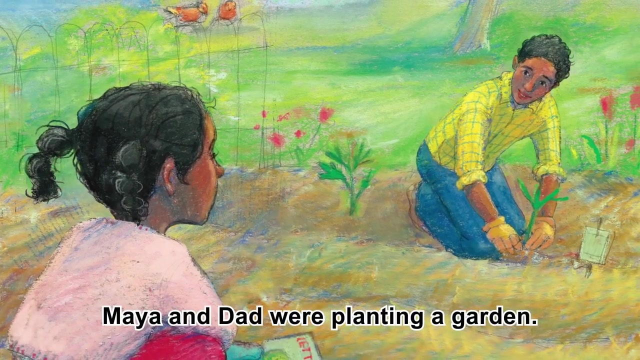 No more apples in the apple tree. But look in the garden. What do you see? There's lettuce and broccoli. Enough for you, enough for me. Maya and Dad were planting a garden. I've put the tomatoes in, said Dad. 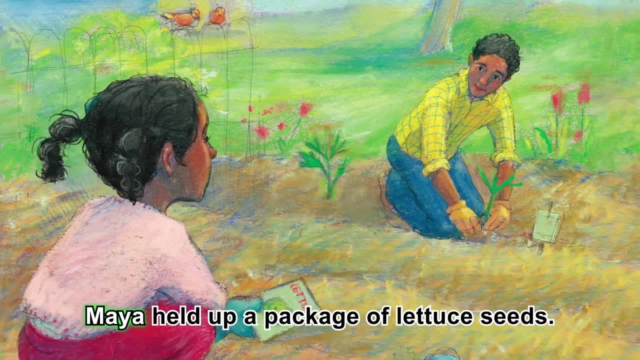 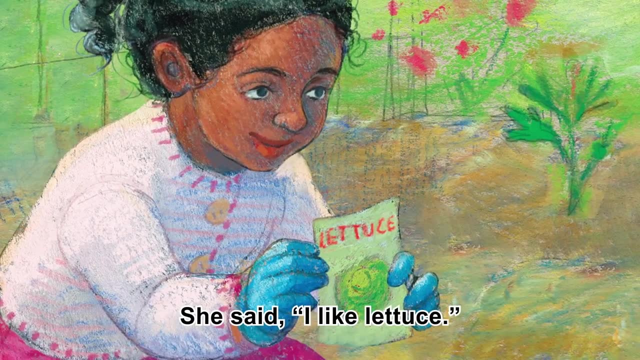 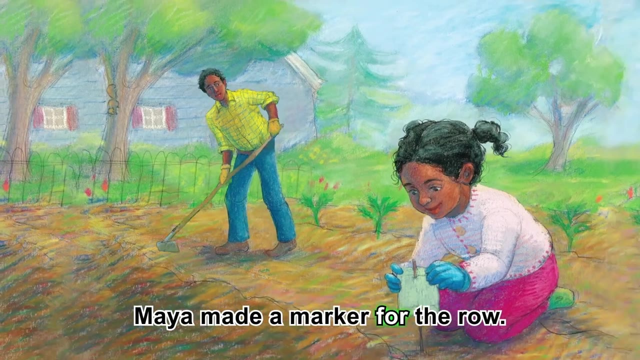 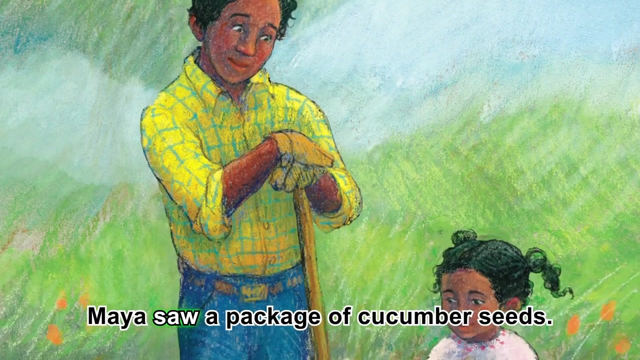 What else do you like? Maya held up a package of lettuce seeds. She said: I like lettuce. While Dad planted the lettuce seeds, Maya made a marker for the row. What else shall we plant, asked Dad. Maya saw a package of cucumber seeds. 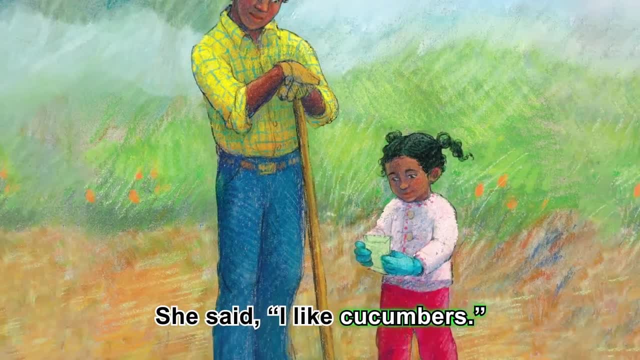 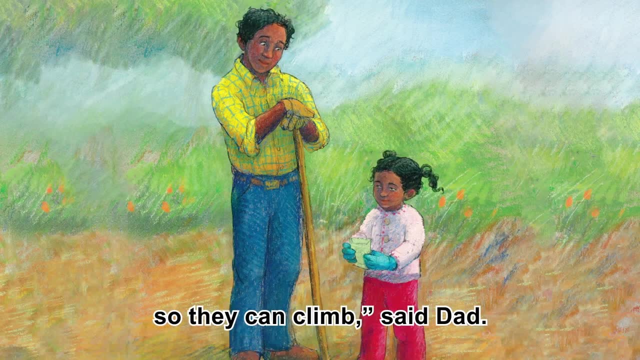 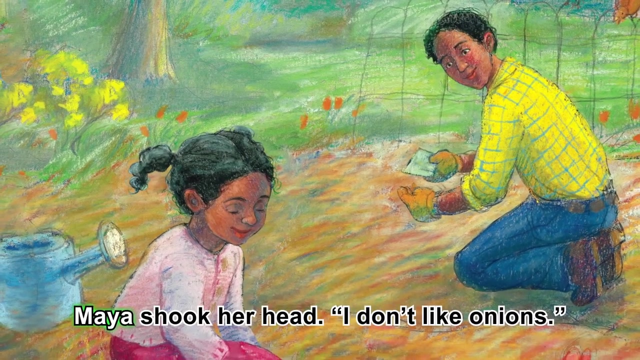 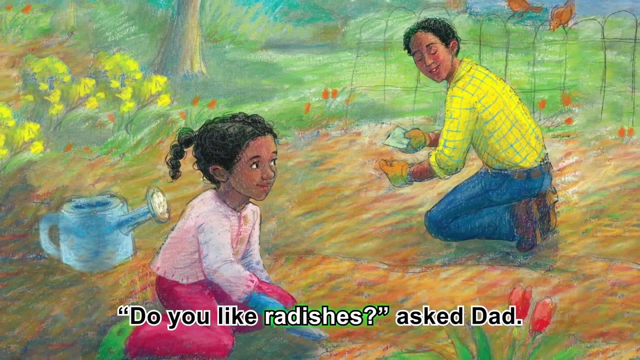 She said: I like cucumbers. Let's plant them by the fence so they can climb, said Dad. Shall we plant some onions, Dad asked. Maya shook her head. I don't like onions. Do you like radishes? asked Dad. 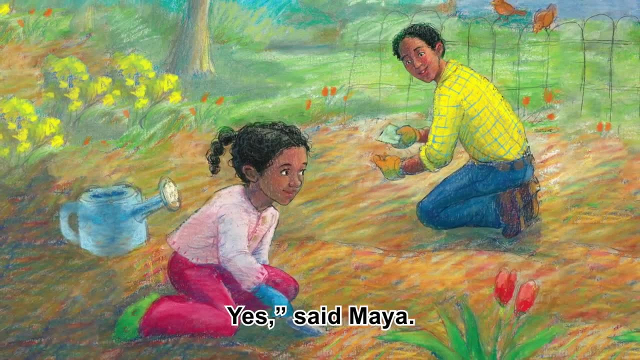 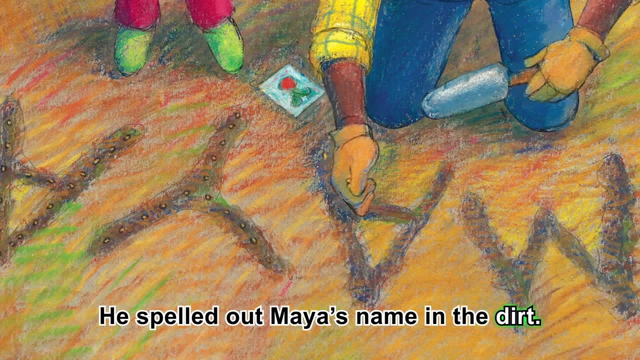 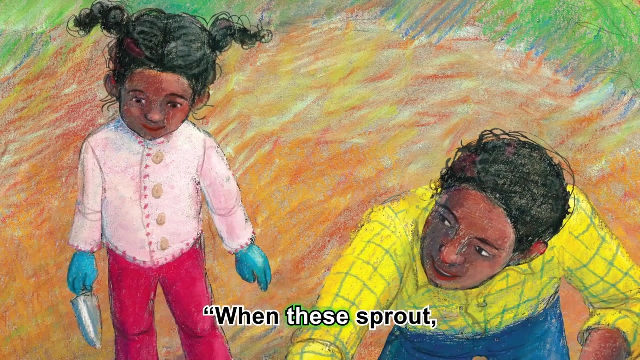 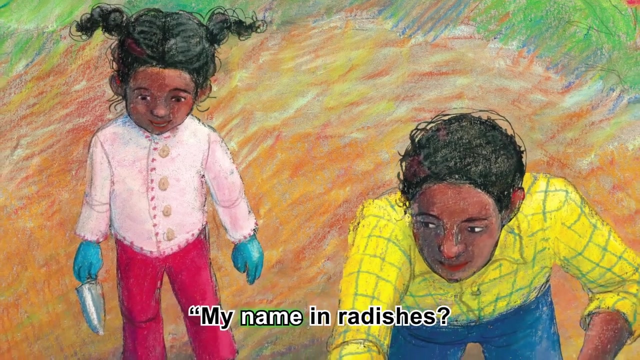 Yes, said Maya. Watch this, said Dad. He spelled out Maya's name in the dirt. Then he sprinkled radish seeds along the letters. When these sprout, you'll have your name in radishes. Maya grinned. My name in radishes. I like it. 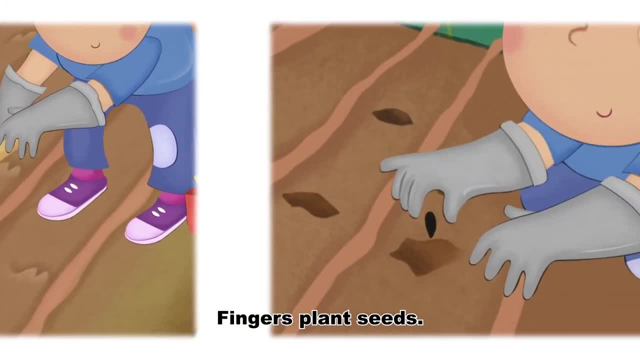 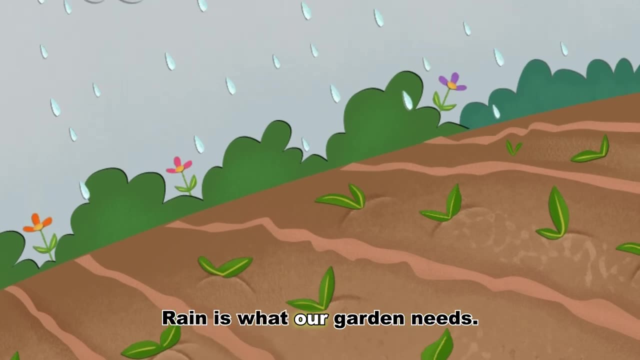 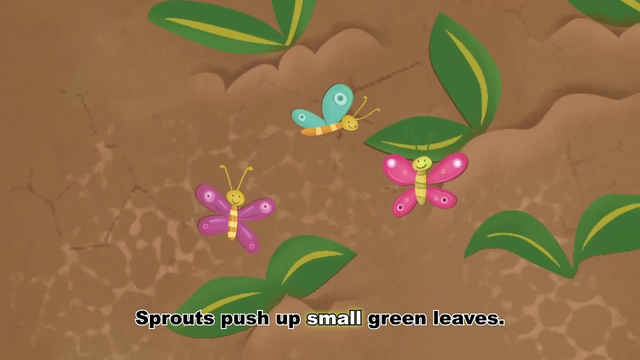 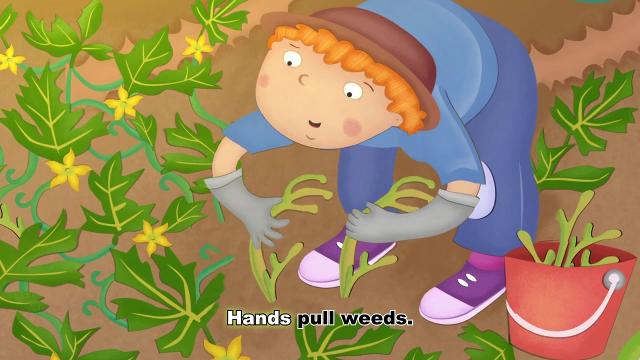 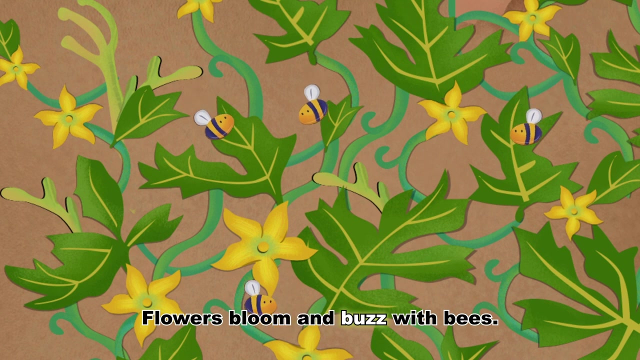 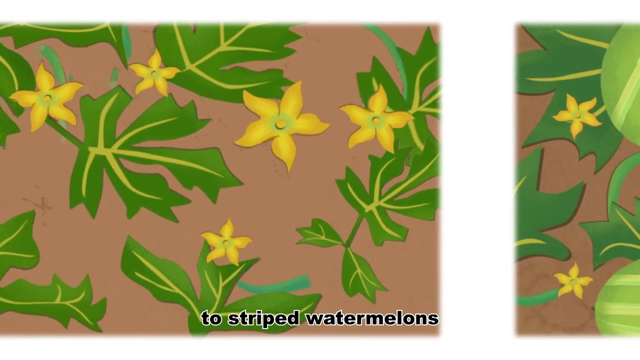 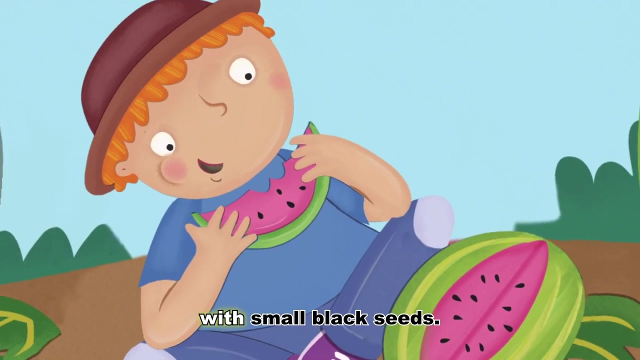 Make rows Fingers, plant seeds. Rain is what our garden needs. Sprouts push up small green leaves. Sunshine warms Hands. pull weeds. Flowers bloom and buzz with bees. Fuzzy vines twine and lead to striped watermelons with small black seeds. 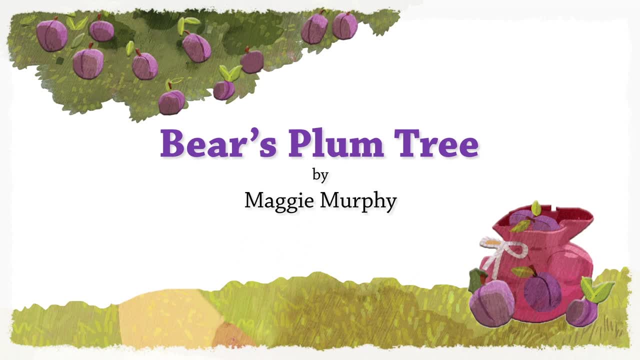 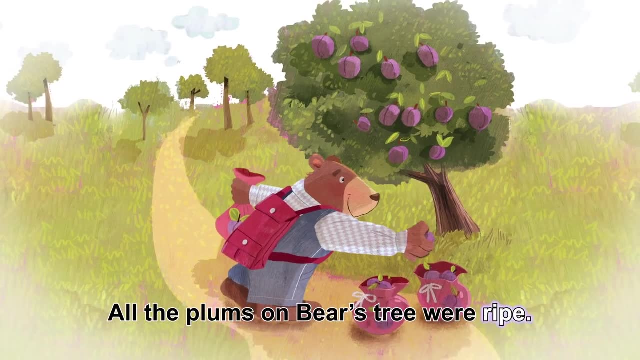 Bear's Plum Tree by Maggie Murphy. Art by Kristin Sora. All the plums on Bear's tree were ripe. All the plums on Bear's tree were ripe. All the plums on Bear's tree were ripe. I'll share these sweet plums with my friends. he said. 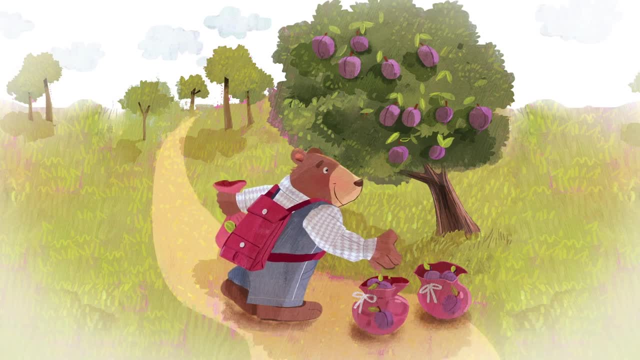 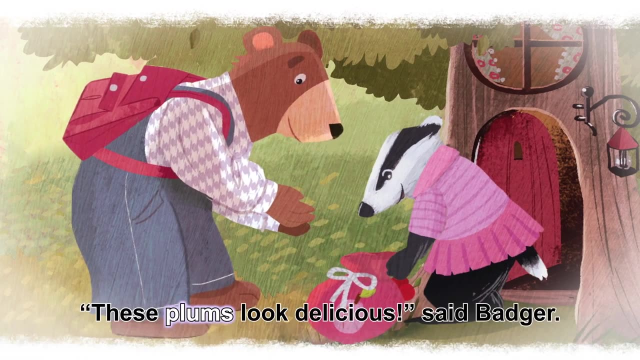 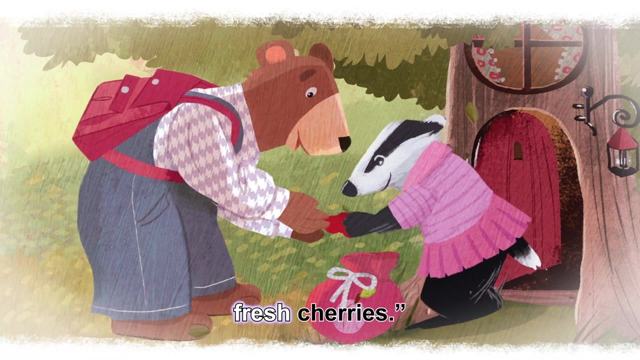 So he filled three bags with plums. Then he strolled off to Badger's house and gave her the first bag. These plums look delicious, said Badger. I have something for you too: Fresh cherries. Thank you, said Bear. 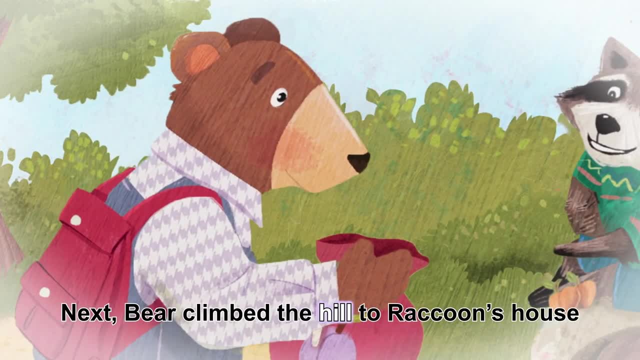 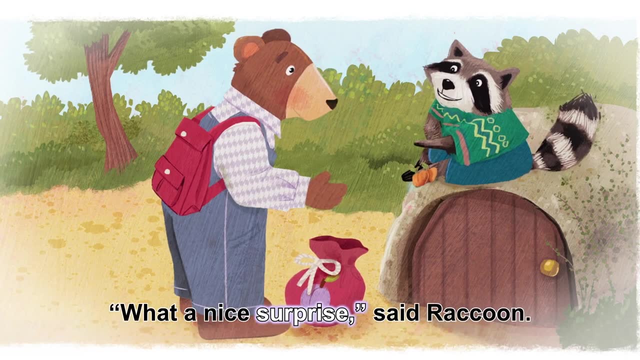 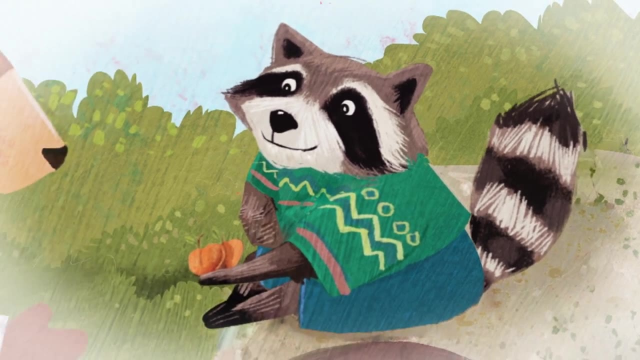 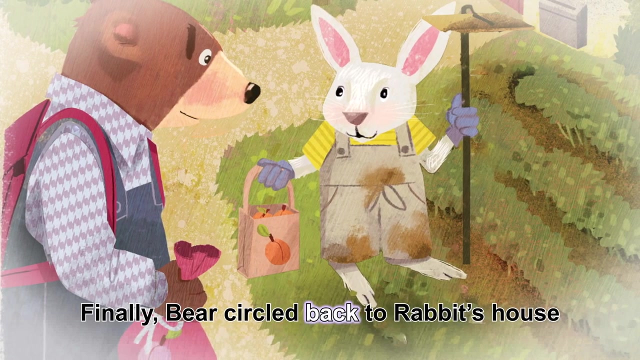 Next, Bear climbed the hill to Raccoon's house and gave him the second bag. What a nice surprise, said Raccoon. I have something for you too, Apricots. Thank you very much, said Bear. Finally, Bear circled back to Rabbit's house. 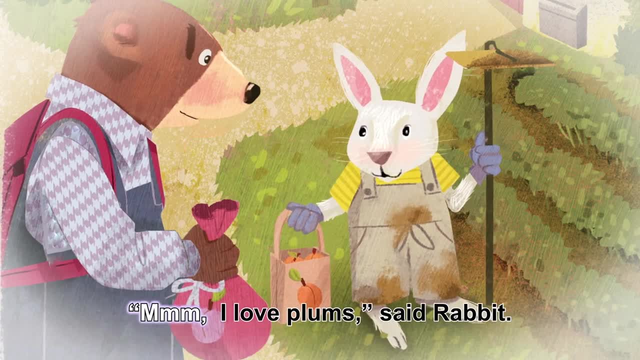 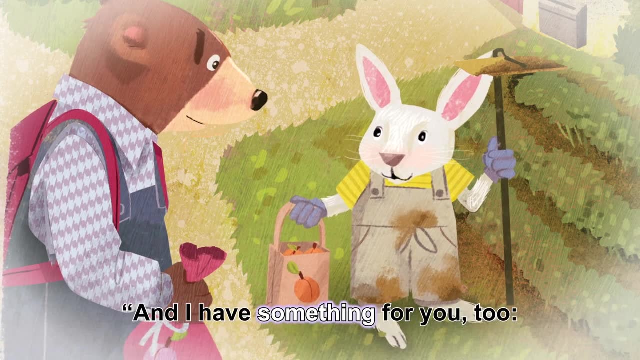 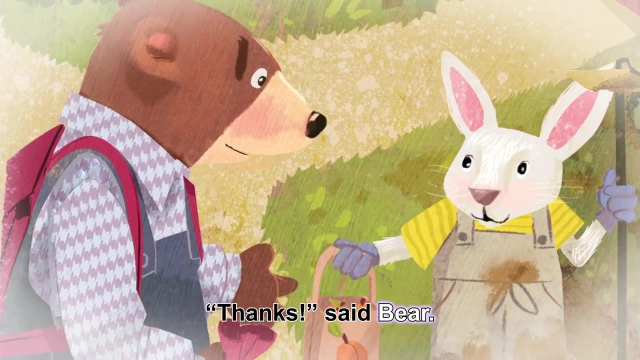 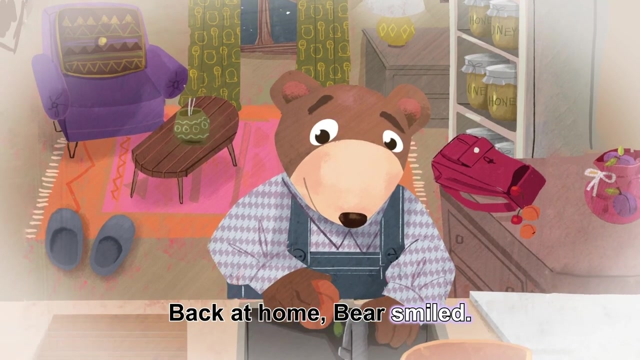 and gave him the third bag. Mmm, I love plums, said Rabbit, And I have something for you too: Peaches from my trees. Thanks, said Bear. I have wonderful friends Back at home. Bear smiled: Now I know just what to eat for supper, he said. 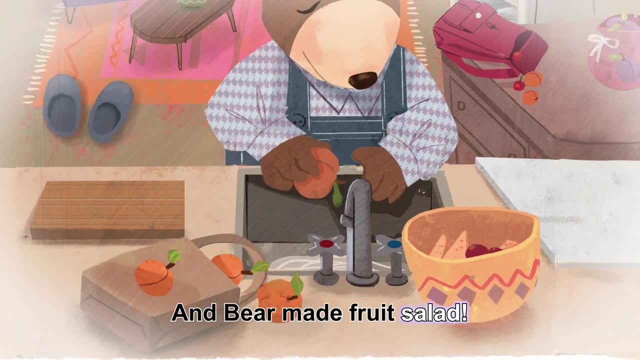 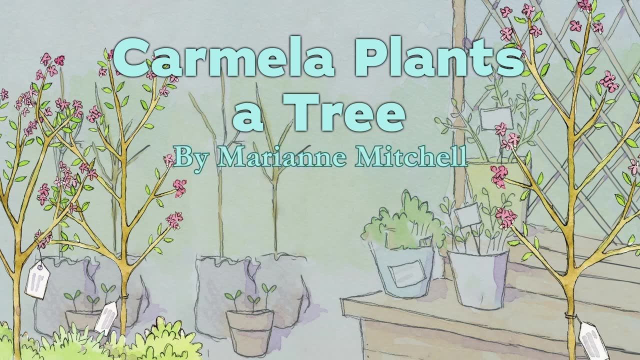 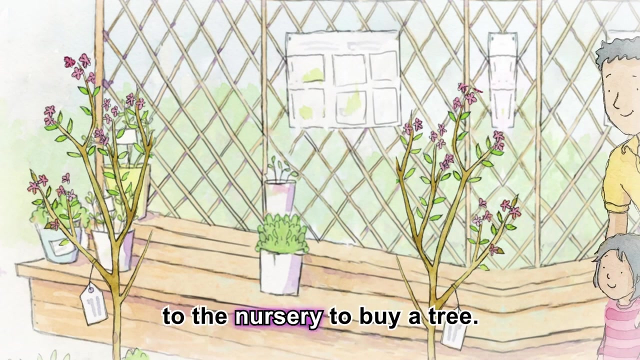 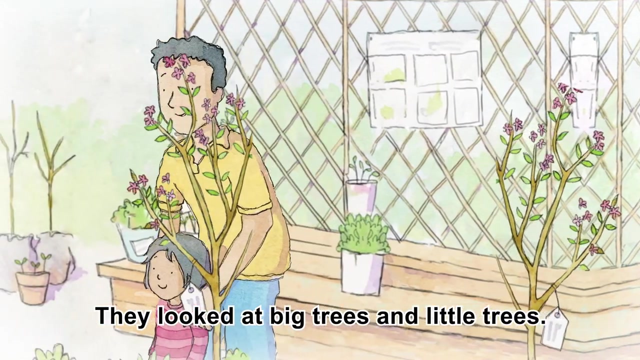 And Bear made breakfast. Bear made fruit salad. Carmela Plants a Tree by Mary Ann Mitchell. Art by Claire Key. Carmela went with Dad to the nursery to buy a tree. They looked at big trees and little trees. Carmela chose one with pretty flowers. 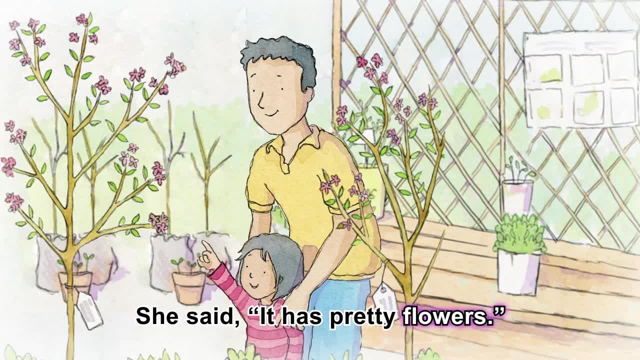 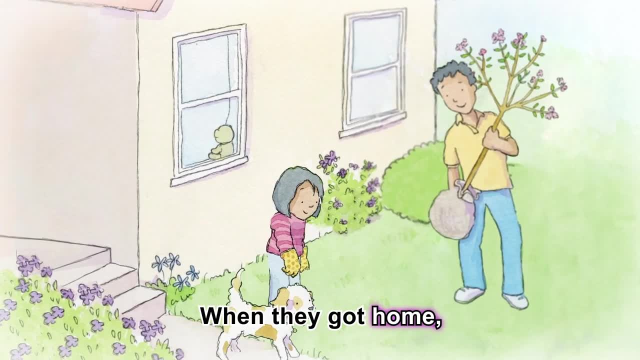 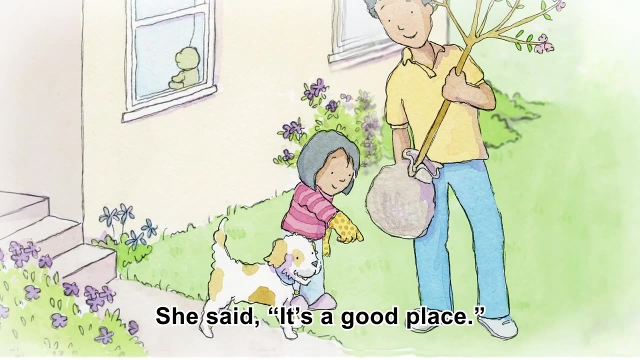 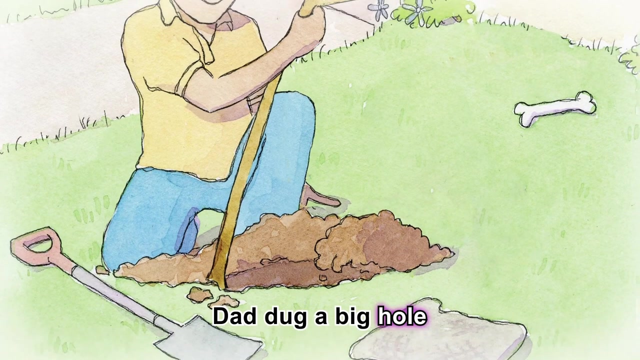 She said It has pretty flowers. Good choice, said Dad. When they got home they looked for a good place to plant the tree. Carmela wanted it near her bedroom window. She said It's a good place. Dad dug a big hole. 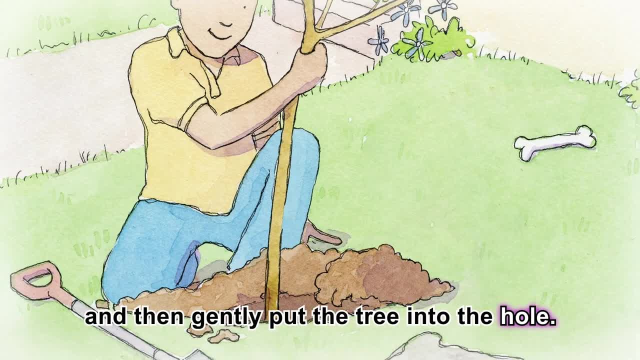 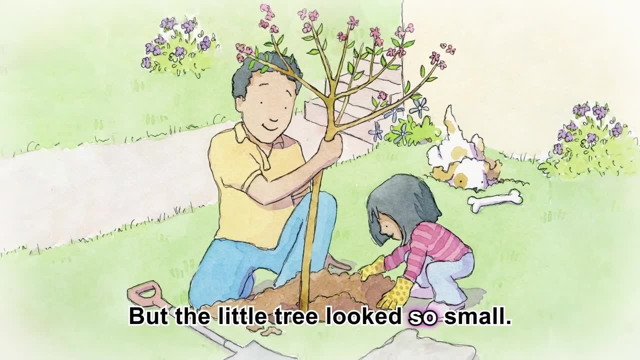 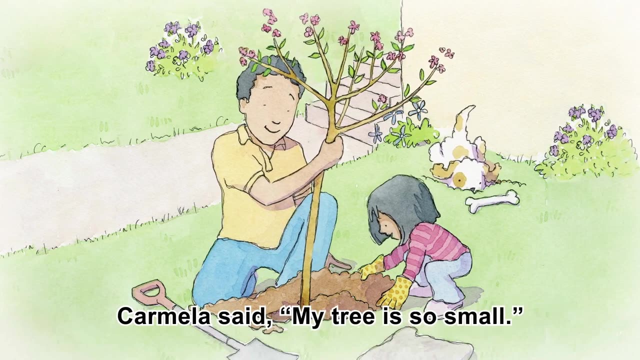 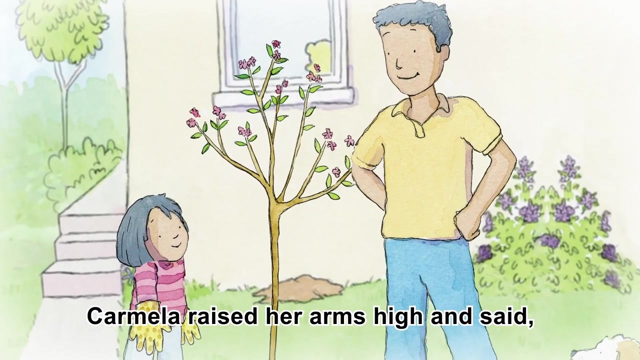 and then gently put the tree into the hole. Carmela helped him fill the hole with dirt, But the little tree looked so small. Carmela said: My tree is so small. Someday it will be big and tall, said Dad. Carmela raised her arms high and said: 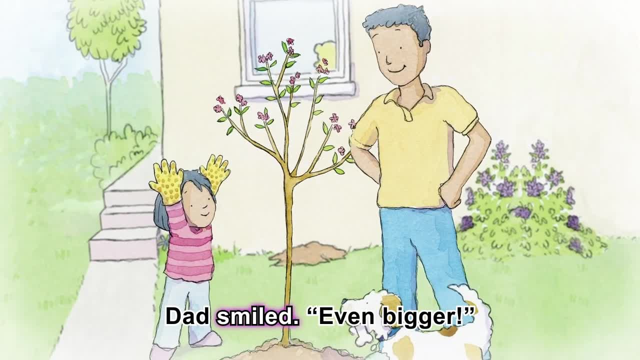 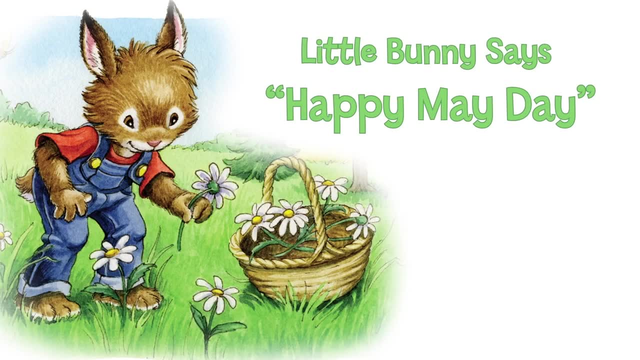 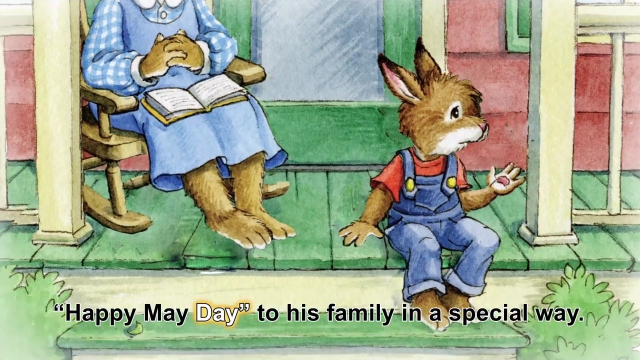 As big as you are. Dad smiled Even bigger. Little Bunny Says Happy May Day by Eileen Spinelli. Art by Rose Mary Berlin. It was May Day and Little Bunny wanted to say Happy May Day to his family in a special way. Granny, what can I do?